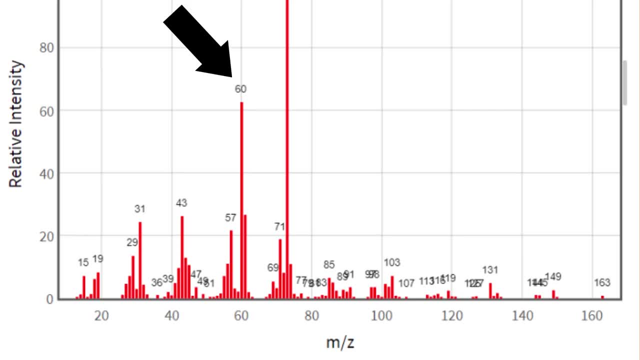 ratio, The length of the bar or the height of the bar, I should say, indicates the relative abundance of that particular ion, the most frequent being assigned as 100.. Modern mass spectrometers can distinguish or resolve ions differing by a single atomic. 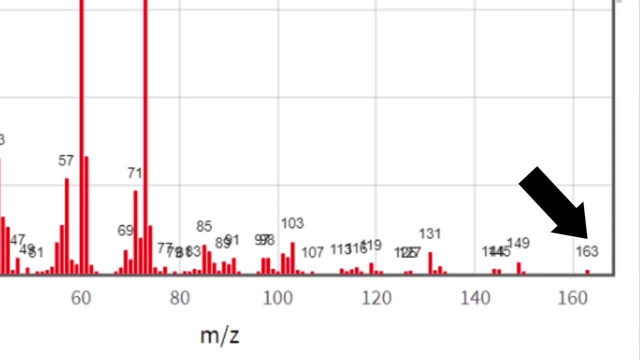 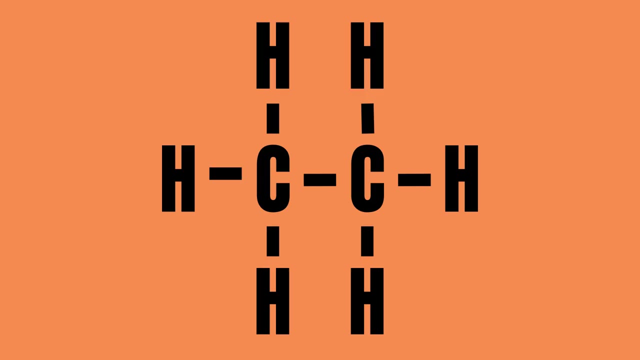 mass unit AMU, The highest mass ion is assumed to be the molecular compound in its entirety, and any lower mass ions are assumed to be fragments from that molecular ion. To decide where this fragmentation has occurred, one needs to consider the strength of the bonds inside of the molecule between the different atoms. 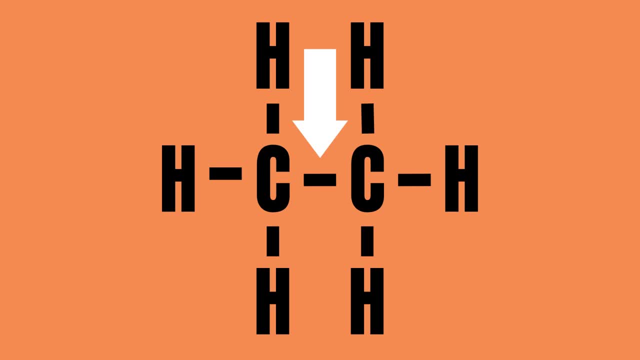 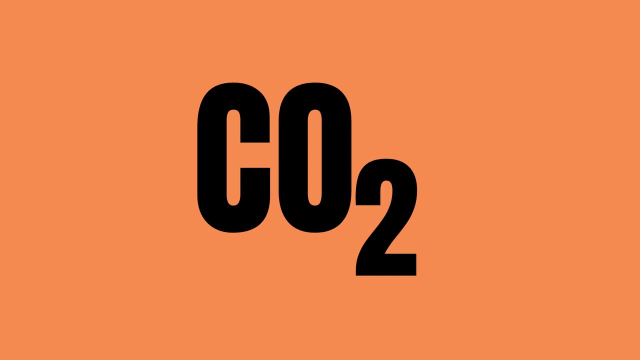 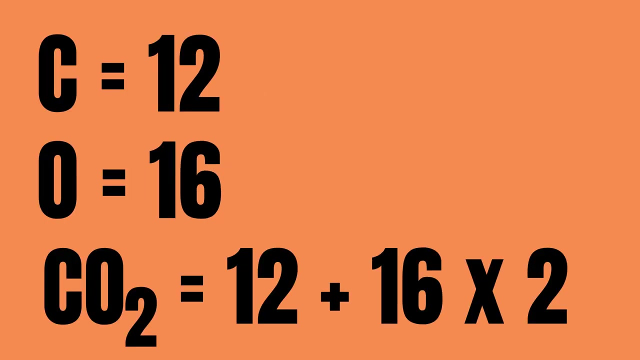 in that molecule. The best way to make sense of all of this is by examining a few examples. Let us start off nice and easy with carbon dioxide, CO2.. Before anything else, it is wise to calculate the total molecular mass of the compound we are interested in. 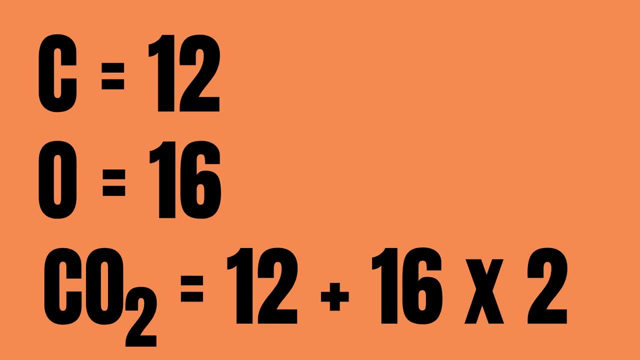 in this case CO2.. Okay so, carbon has a molecular mass of 12, AMU, and oxygen has a molecular mass of 16.. We also know that we have two oxygen atoms in CO2, so therefore, to calculate the total AMU, 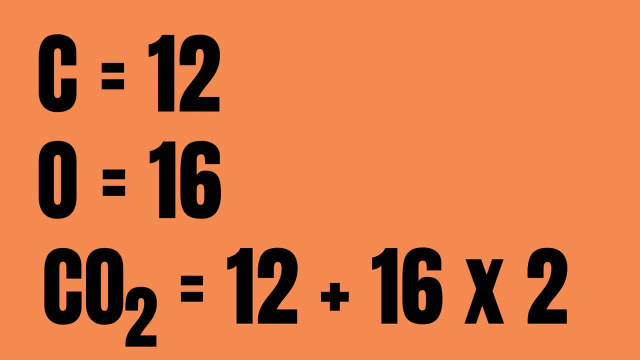 we have 12 plus 16 times 2. This comes out at 44 AMU. This means that what we are going to expect to see is that the bar for CO2 is less than or equal to the total AMU, which is less than or equal. 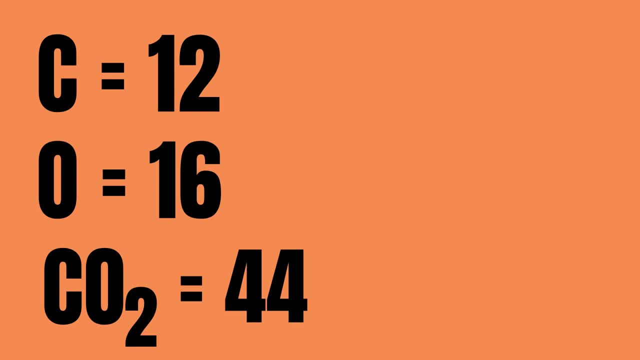 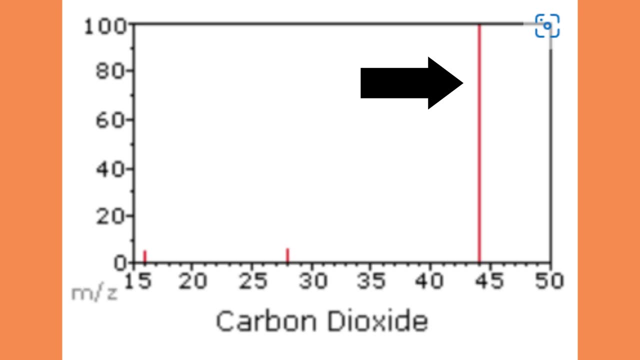 to the total AMU and the bar furthest to the right, the largest one is going to be 44 AMU, And would you look at that? so it is. Second, in order to figure out how the ionization process might break up the compound, let us take a look at its chemical bonds. 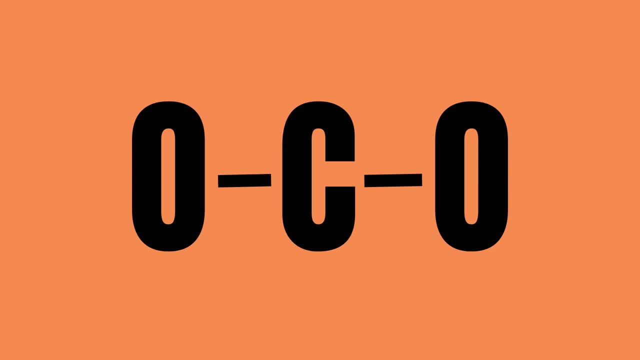 Carbon dioxide is quite simple. it's simply a carbon with an oxygen on both sides of it. In other words, there's really only two ways to split this molecule: either you split the bond between the oxygen and the carbon on the left side. 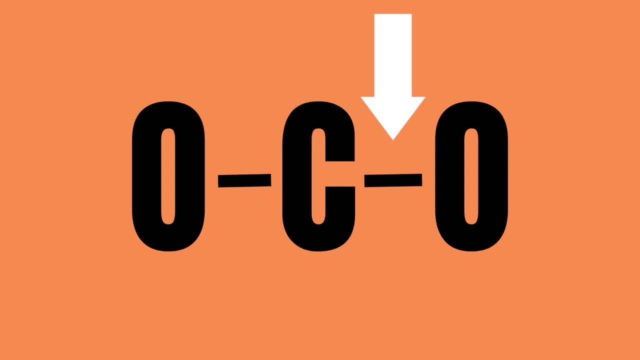 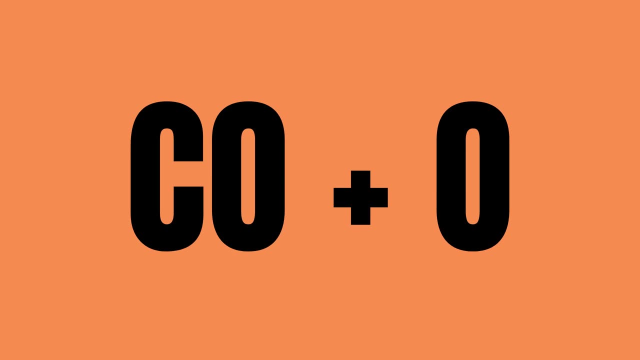 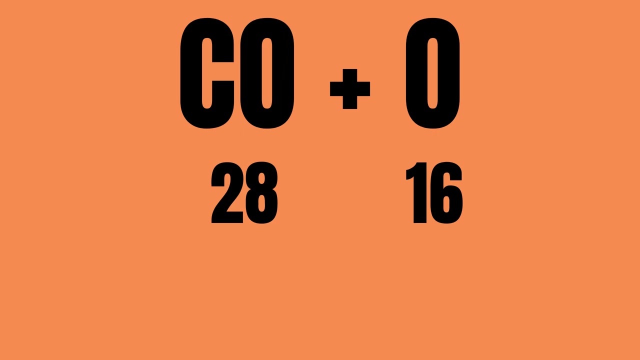 or then you split it on the right side. In either one of these two cases, the result is going to be the same, Namely we're going to be left with a CO plus an oxygen, meaning that the molecular masses of these two compounds is going to be 28,, again 12 plus 16, and 16, which 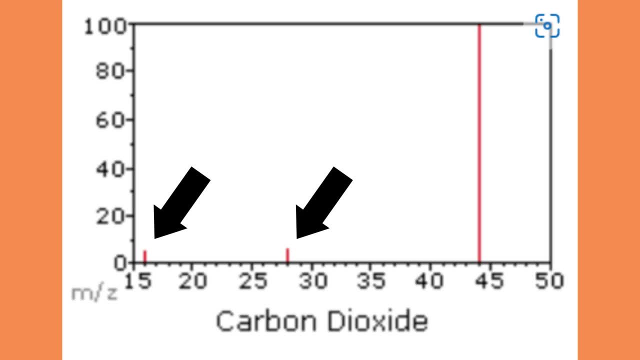 is just oxygen 16.. And when we look at the graph, that is exactly right. In addition, we can infer that the complete carbon dioxide molecule is very stable. it's even the most stable, since it has the highest relative abundance. Okay, let us do one more example, this time using propane C3H8.. 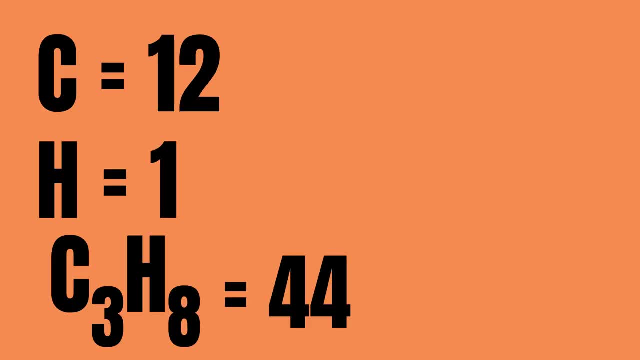 First we will again calculate the total molecular mass of the compound. Here again we have carbon, which has a molecular mass of 12, and we have hydrogen, which has a molecular mass of 12.. And we have hydrogen which has a molecular mass of 1.. 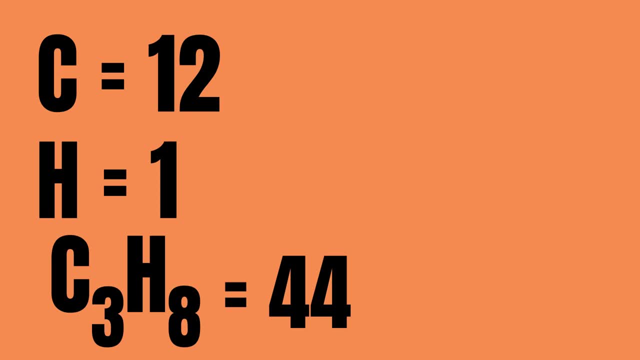 So we have 3 carbons 12 times 3, plus 8 hydrogens 1 times 8.. This results in a total of also 44 amu. So again, this is what we're going to expect: the staple furthest to the right or the largest one to equal 44.. 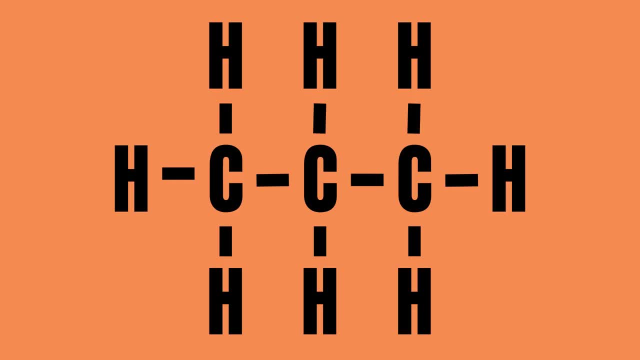 And look at that it does. Then, second, we're going to look at the chemical bonds. So here we have CH3 bonded to CH2, bonded to CH3, and each of these carbon atoms are also bonded to their respective hydrogens, as you can see in the picture. 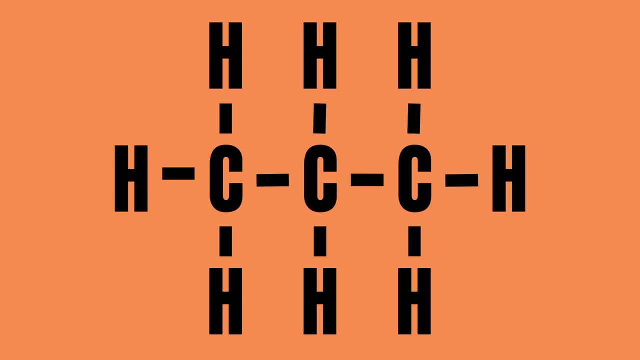 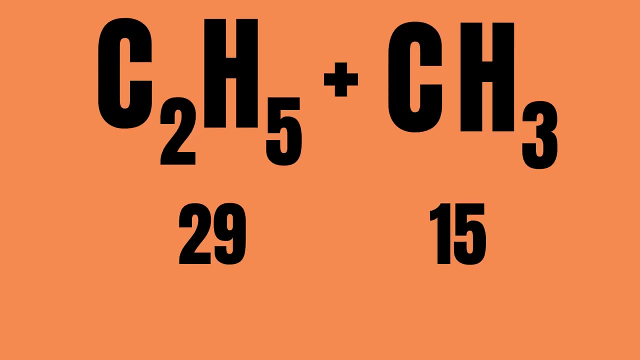 So how do we think that this is going to break up? Well, one sure guess is probably that the bonds between the carbon in the middle and the carbons on the side, those are probably going to break. That would leave us with CH2 to CH3, which has a total molecular mass of 29,. 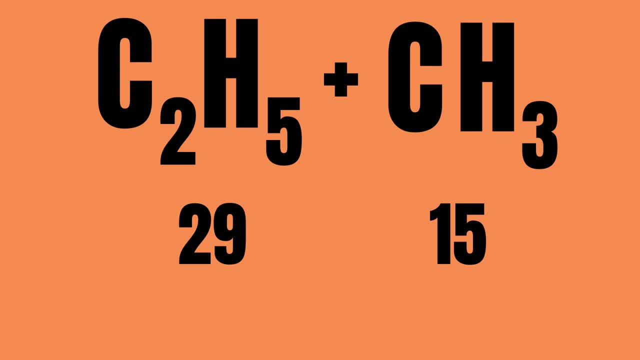 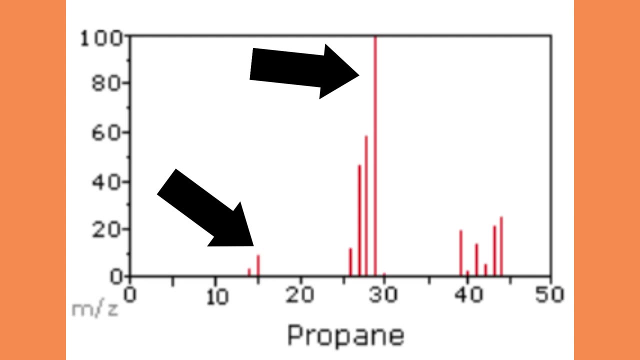 and an alone CH3, which has a molecular mass of 15.. But now, if we look at the graph, this is true, We can find those here and they are the two most abundant ones, or not the two most abundant ones. 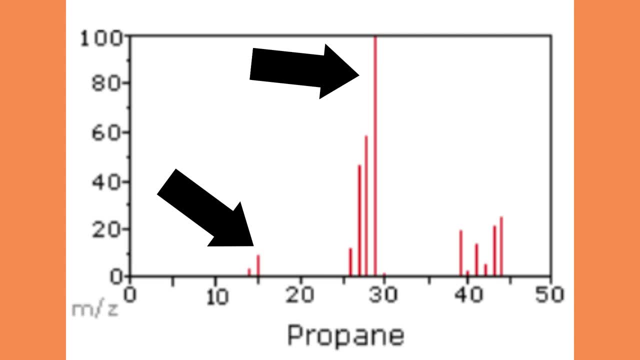 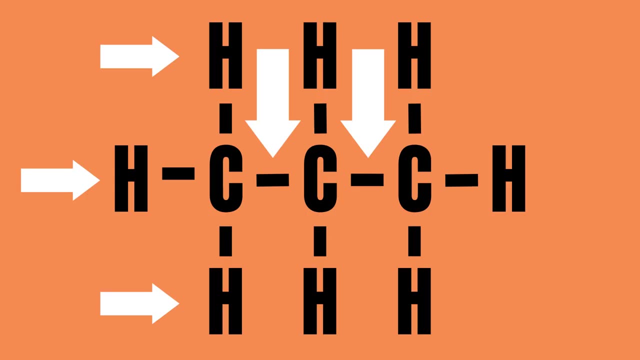 CH3 isn't that abundant, but the 29 definitely is The CH2 to CH3. That's very abundant. But what about all of these other lines? Well, these hydrogens can be knocked off as well. In addition, the bond between two of these carbons can be broken. 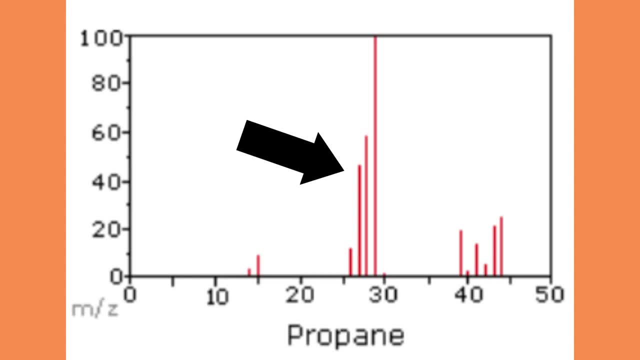 and then a hydrogen can be knocked off as well. So in addition to what we saw there earlier, we can also have it so that first these two carbons, the bond between them, get broken, and then one or several of their hydrogens in addition also get knocked off.